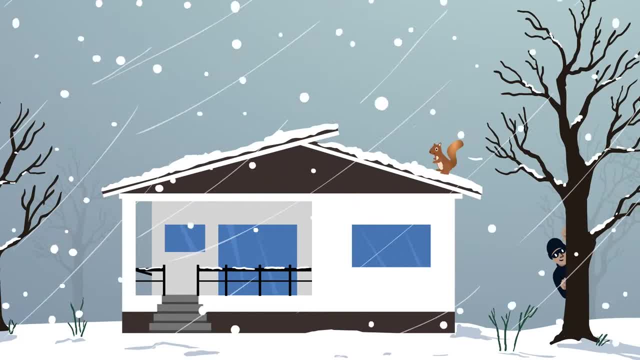 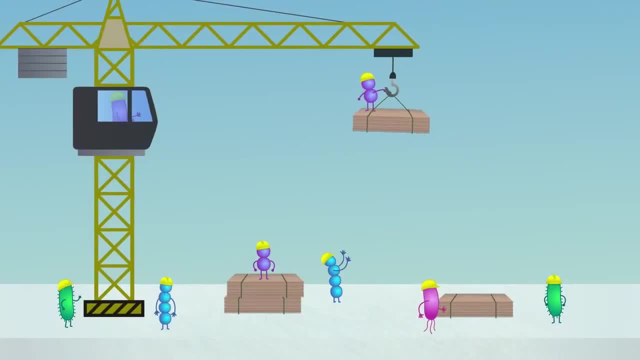 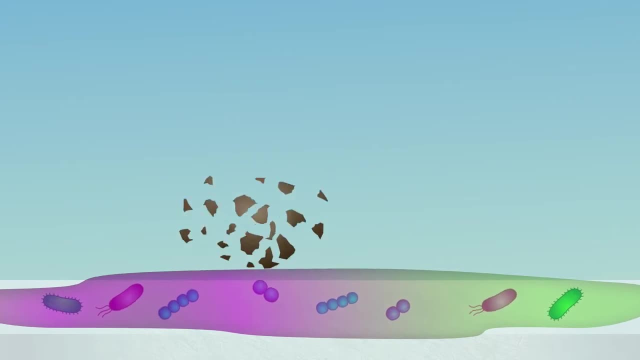 burglars by building houses and places to store food and water. This has increased their chances of survival. Microorganisms have also adapted to natural threats in similar ways. While bacteria don't build homes, they do construct biofilms that serve as very strong protections against dehydration and physical or chemical attacks. 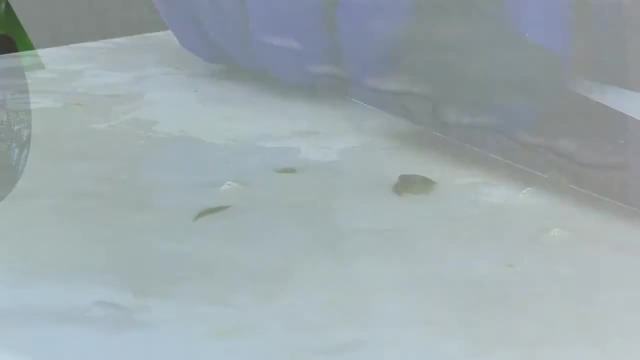 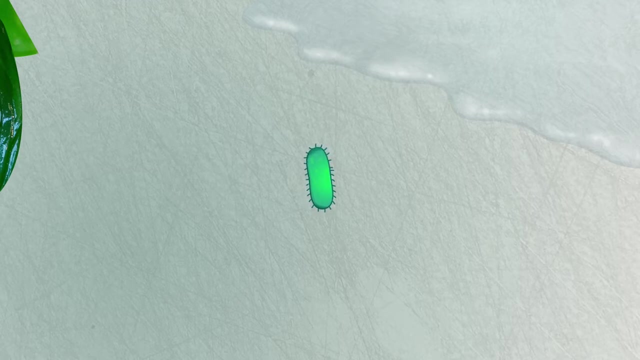 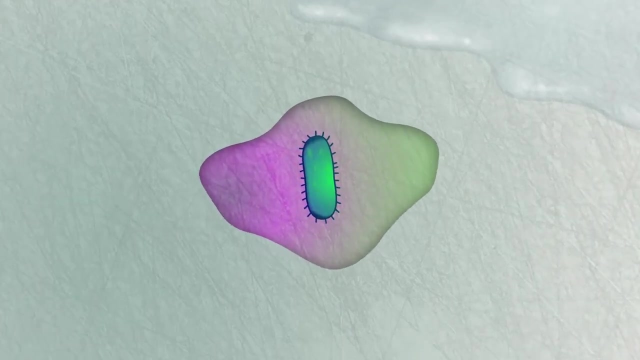 Here's how they do it: The bacteria first find a suitable location that offers life's basic needs- food, water, nice temperatures. Then they start secreting a slimy substance composed mostly of sugars and proteins. Soon, these sugars and proteins turn into what we call biofilm, because it is actually a 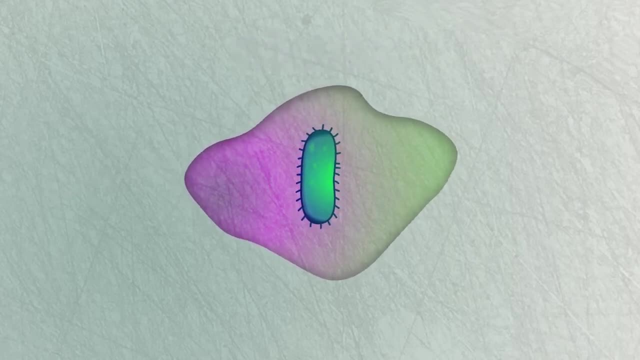 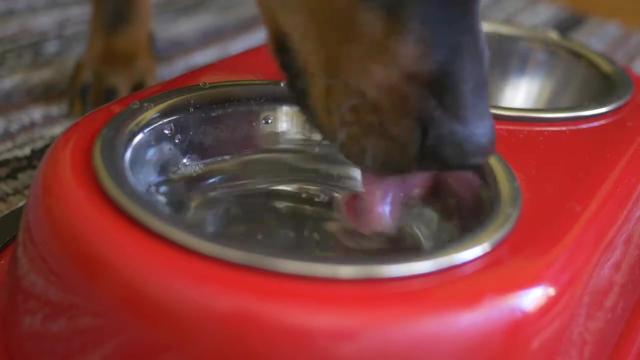 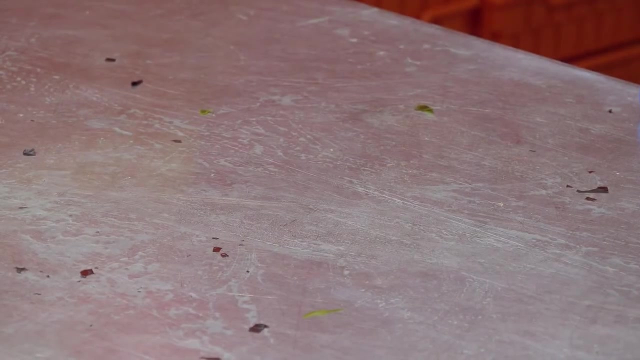 living film of protection for the bacteria. Biofilms can grow everywhere, from the plaque on your teeth to the slime at the bottom of your dog's water bowl, To that yucky stuff that grows between your shower lining and the bathtub. Wet surfaces such as those found in processing plants are prime locations for the formation. 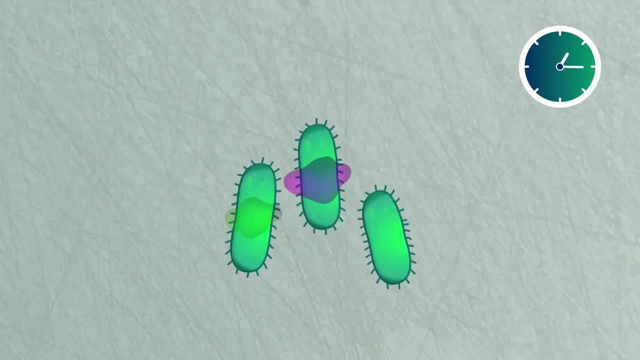 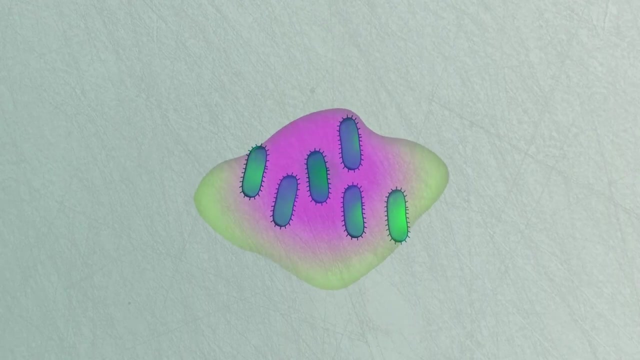 of biofilm. Bacteria and pathogens can start attaching to surfaces in only 30 minutes And within only 8 hours the protective biofilm can be firmly established. As the bacteria continue secreting their slimy sugars and proteins, the biofilm becomes more. 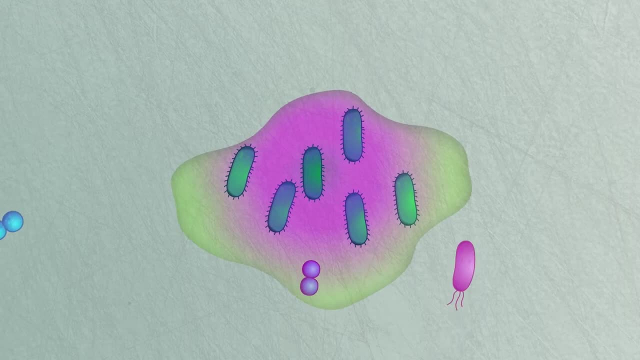 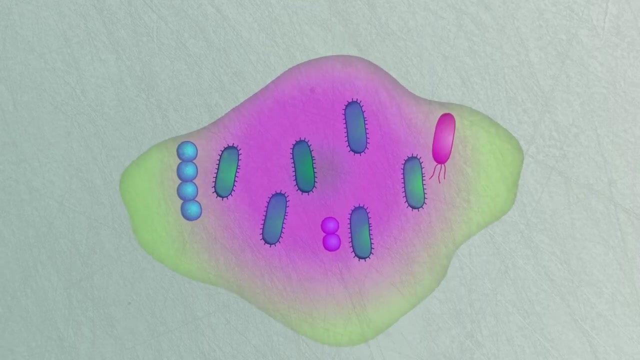 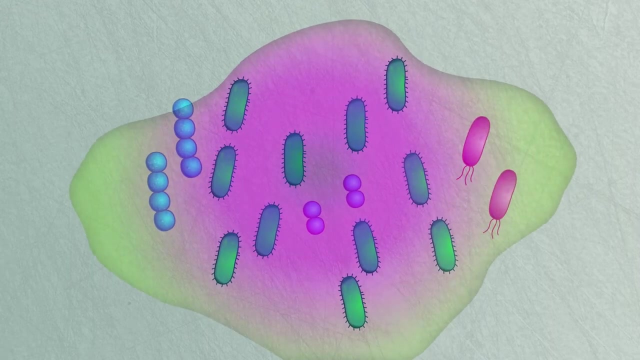 and more established. Other bacteria, even from other species, may join the community, Creating an even bigger, stronger and harder to remove biofilm, protecting the entire community. Once established, the chemical bonds within the biofilm become so strong it's extremely. 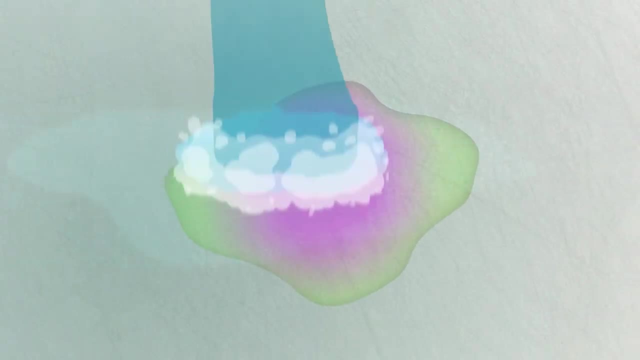 difficult to destroy. Unfortunately, cleaning techniques like regular scrubbing that would normally get rid of pre-living bacteria called planktonic bacteria, are usually not strong enough to get rid of the slimy biofilm. Instead, you need to get rid of the slimy bacteria. 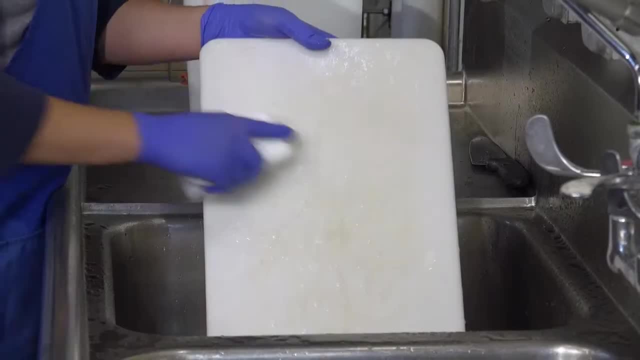 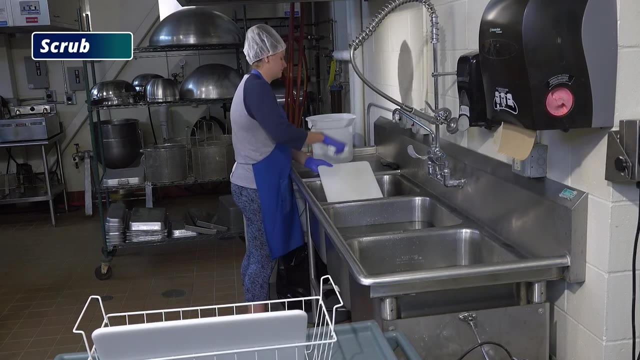 You need to get rid of the slimy bacteria. You need an extremely vigorous physical treatment, In other words, lots of elbow grease. You start by scrubbing vigorously with a brush. Unfortunately, scrubbing alone will not completely remove the biofilm.